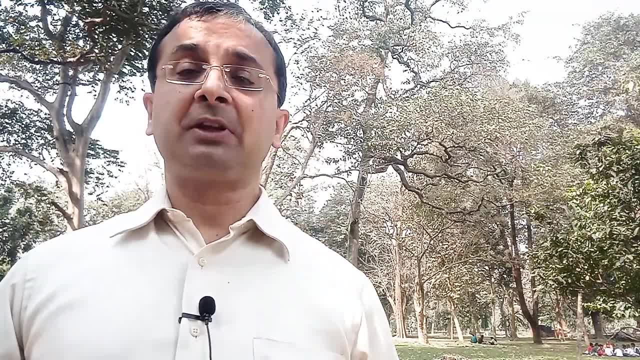 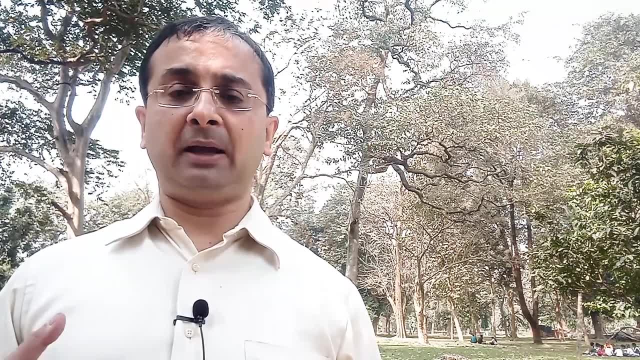 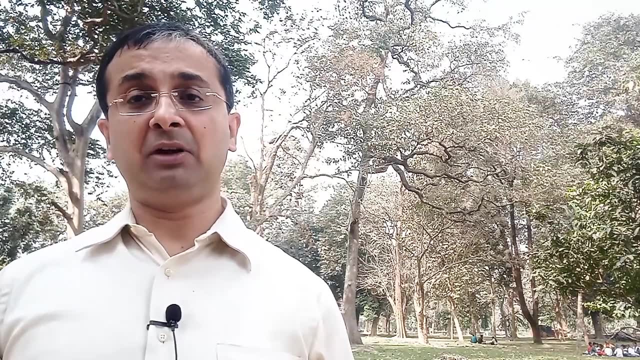 like to give you. it decomposes things and makes it easier. So if you're willing to go as a data scientist, please do learn linear algebra. Do the all mathematics of linear algebra exercises. Do not skip anything, because my recent visit to Bangalore and other places, I found that those people who 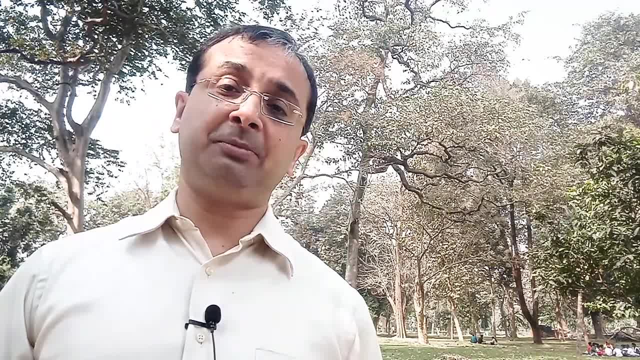 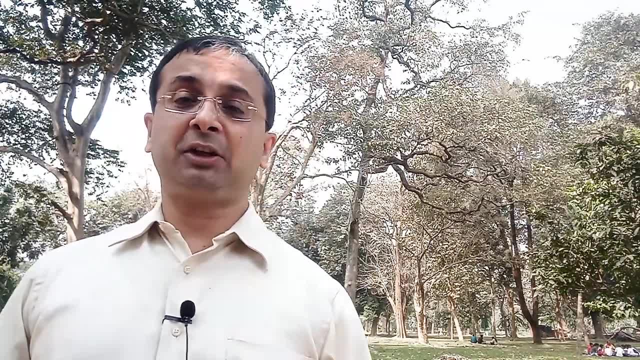 are really working as a data scientist. they have linear algebra quite well exercised and they really know what is linear algebra. The second thing which comes is what is linear algebra? It's called computer graphics. You all know there's a raster mode and there is a GIF, bitmap and other. 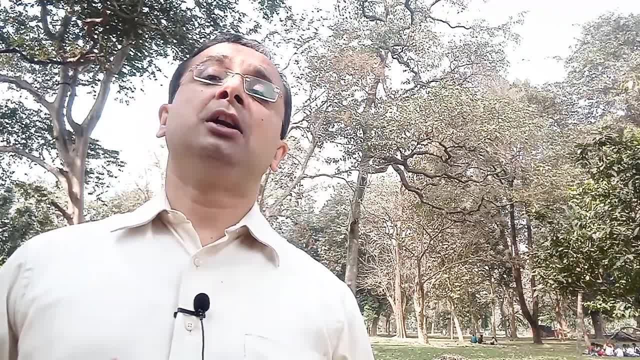 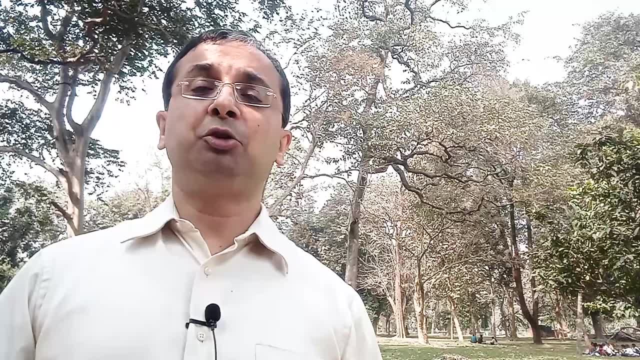 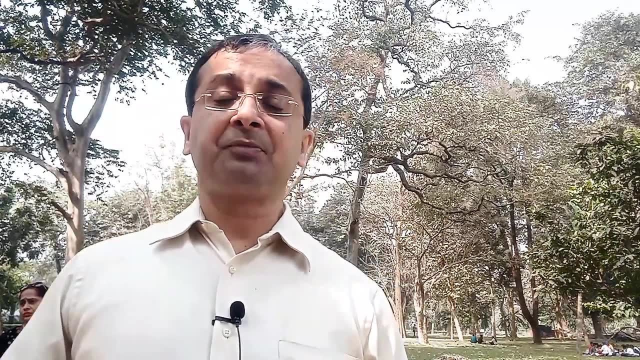 different types of graphics. which happens Now. what happens is that when you are using a graphics, and you are using that in order to what I would say, to skew it, to stretch it, to flip it, and you can rotate it, you can have a reflexive angle. all these are being done through linear algebra. 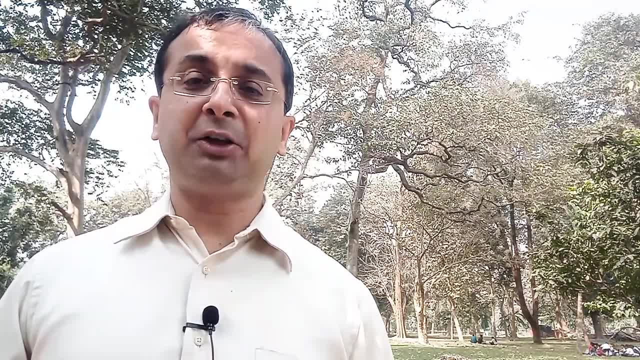 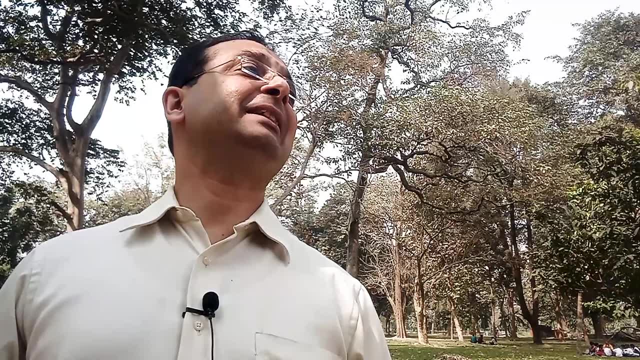 Now, what I'm trying to tell is that when you're doing with the linear algebra, you deal with numbers- huge. that is one part. Also, you deal with a lot of graphics. Now I mean to say there is some kind of a cryptography, there's some kind of a way. 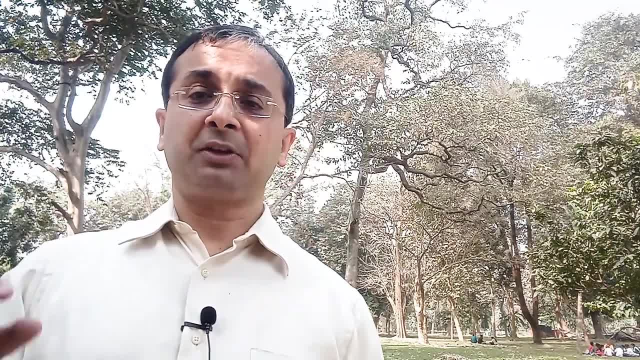 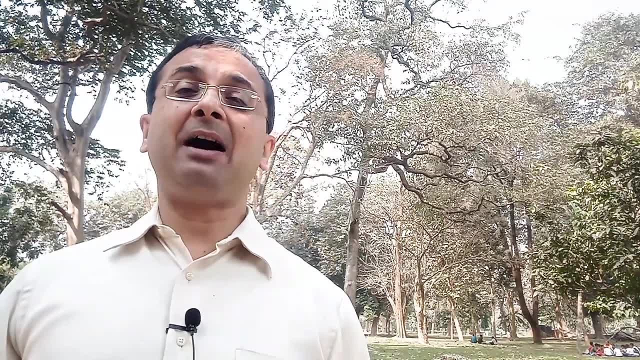 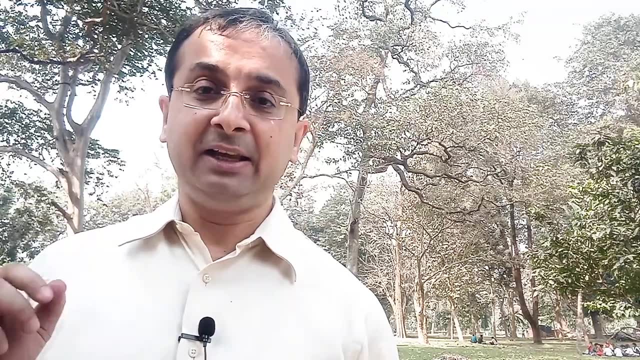 in which you can really codify the data. So the first line would read cat and the second line would maybe read milk. So a way of codifying the data is also done through linear algebra. So first, if you're willing to go as a data scientist, it is the. 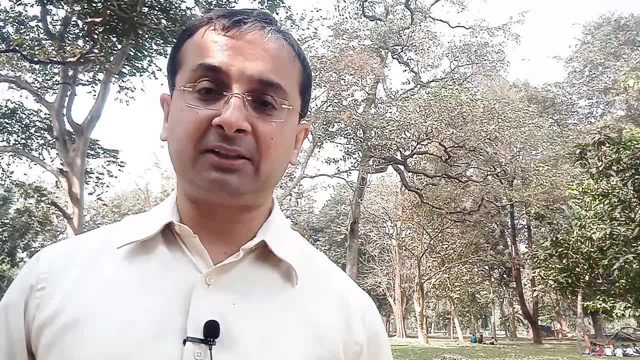 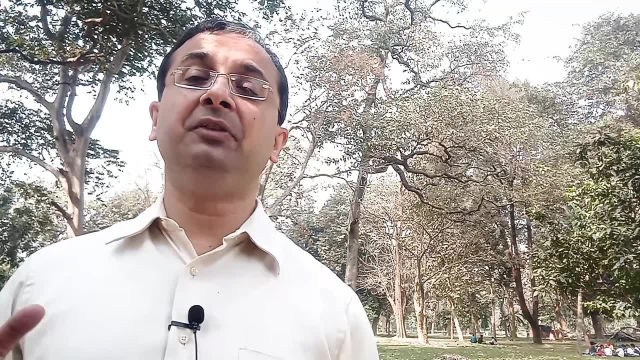 discipline for you. If you want to go into image consultancy, I'm going to say not image consultancy, but deal with images, computers, graphics, etcetera. the definitely you have to deal with what is called linear algebra. The third thing which comes across: 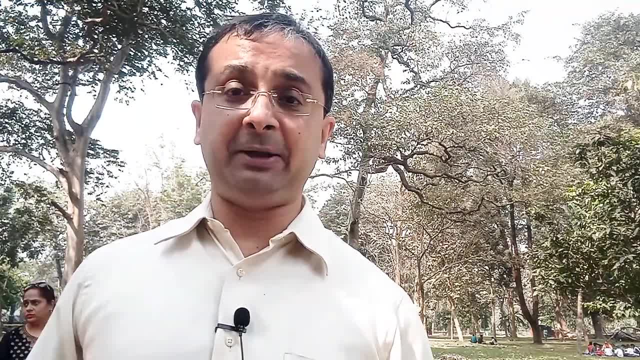 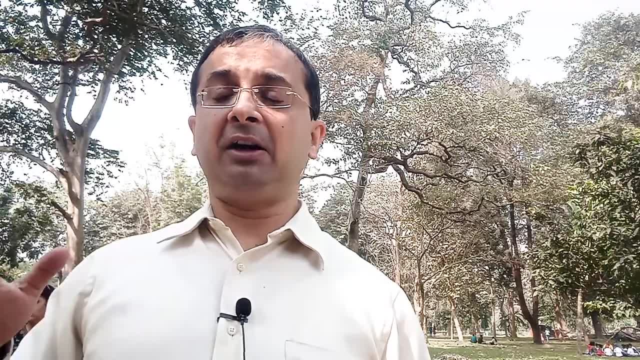 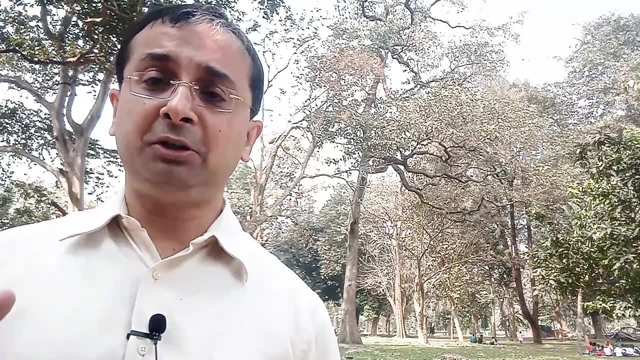 is that linear algebra is also used in computer gaming. Say, for example, I'm firing somebody and there's a coordinate right, Then how these coordinates are being arranged, If you arrange one coordinate with the other, If you are arranging these things one part of the other, and so then linear algebra is equally important, because linear algebra deals. 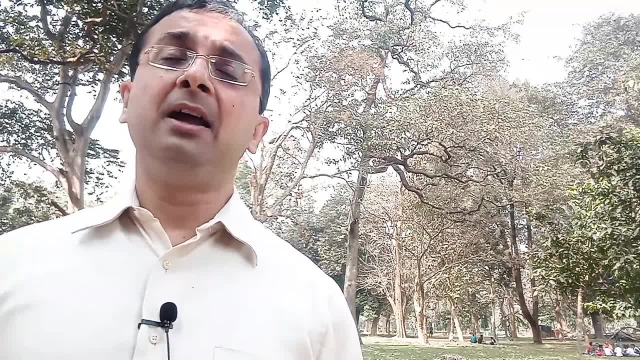 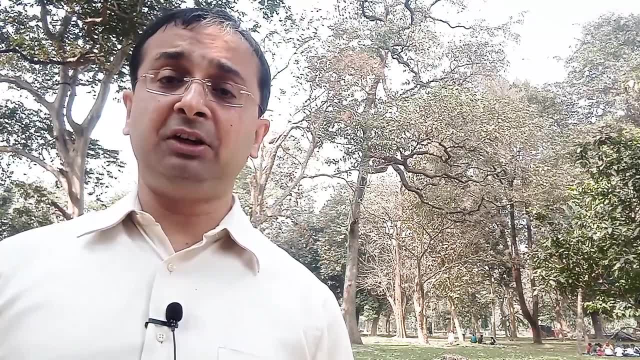 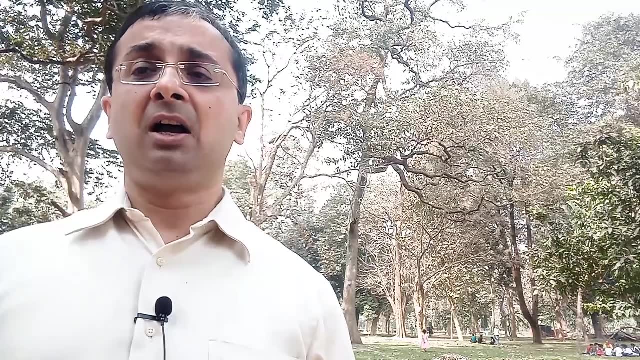 with graphics and vectors come into the play. apart from that, there are a lot of other usage in linear algebra. for example, for deep learning and for machine learning, linear algebra is very important. numpy is also being used. using linear algebra, machine learning is being used a lot of. 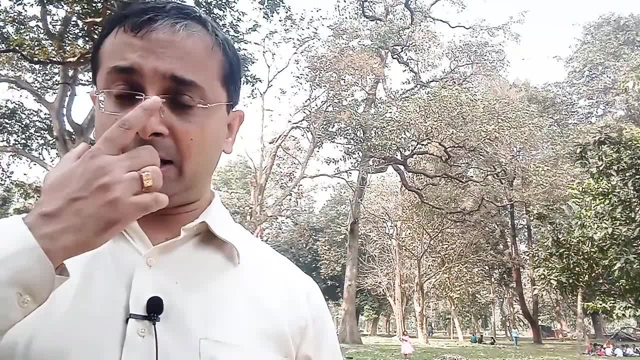 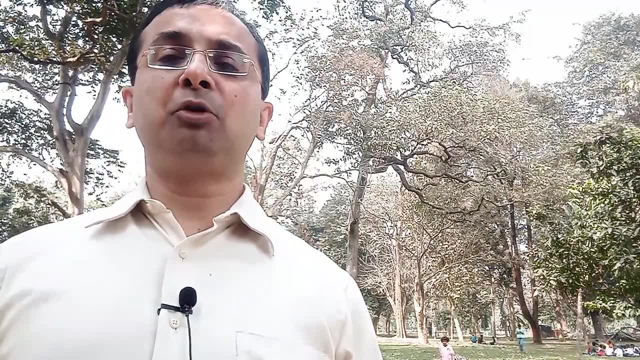 other things are being used. so just to summarize in all- i don't want to make the video too long- there are practical applications. you must have seen a lot of practical application. but, most importantly, linear algebra gives you a job as a data scientist, gives you a good secure. 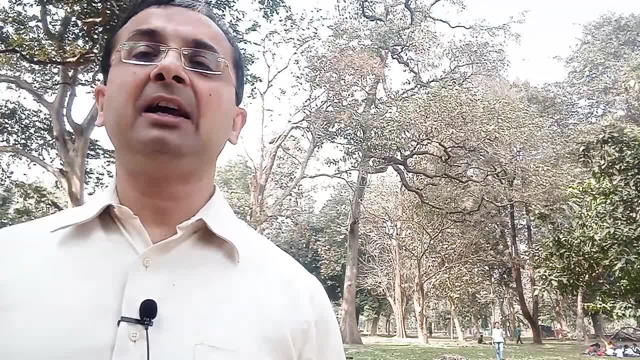 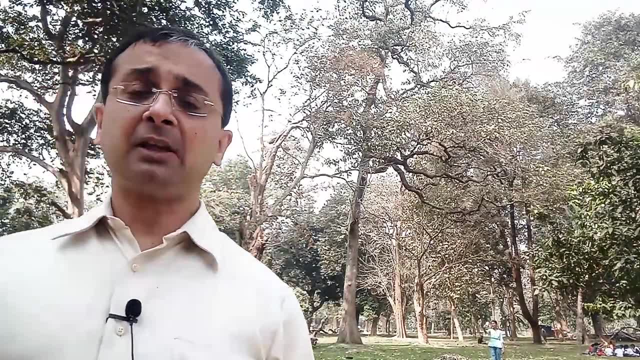 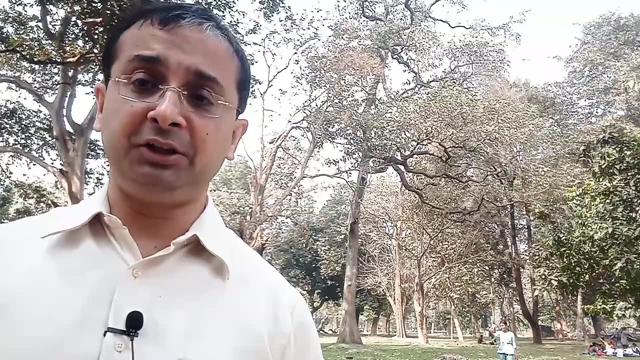 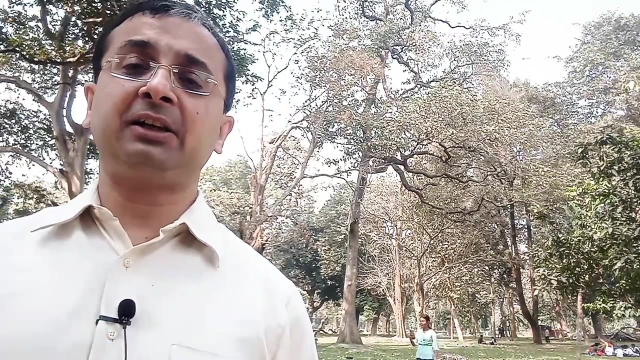 job into image processing, into deep learning and, if you're willing to go into number, into into machine learning. also remember, nowadays we are talking a lot about cyber, secure security, quantum entanglement. these also use linear algebra, because linear algebra is an efficient way to codify the data. i mean to say you make the data in such a way that it is very 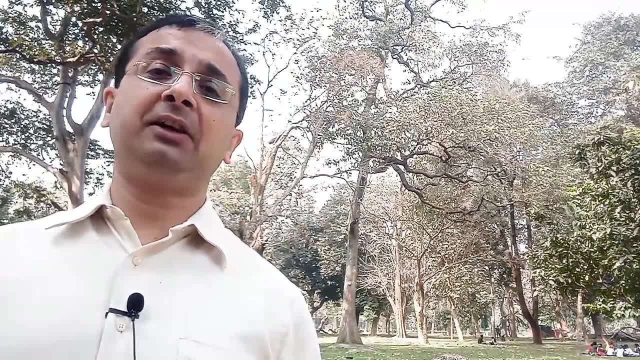 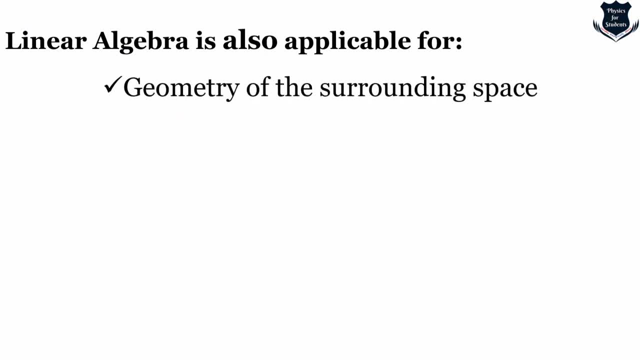 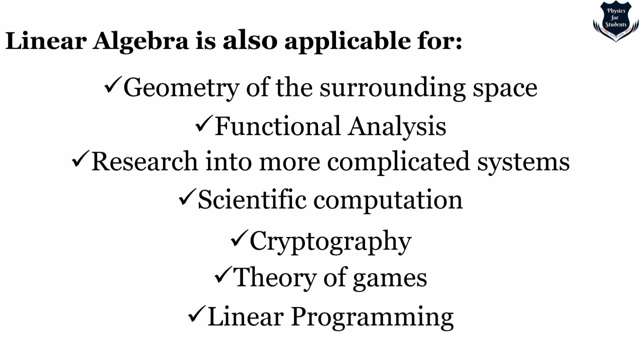 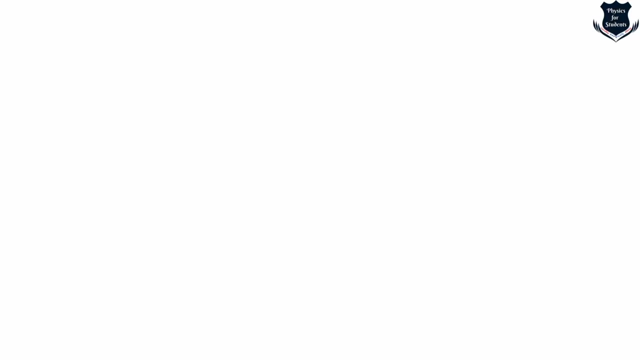 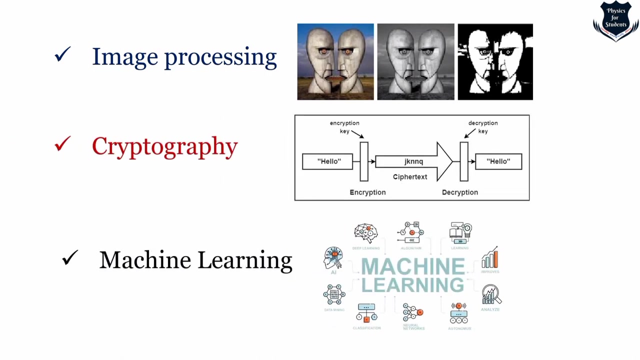 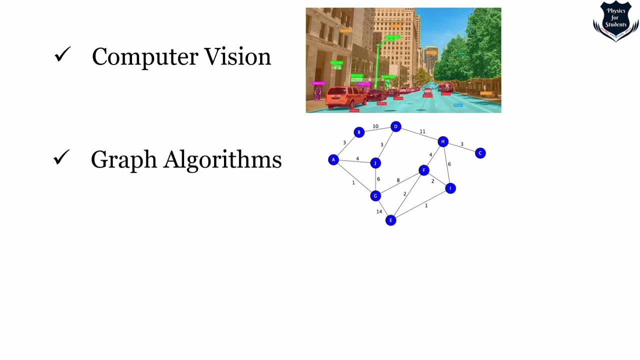 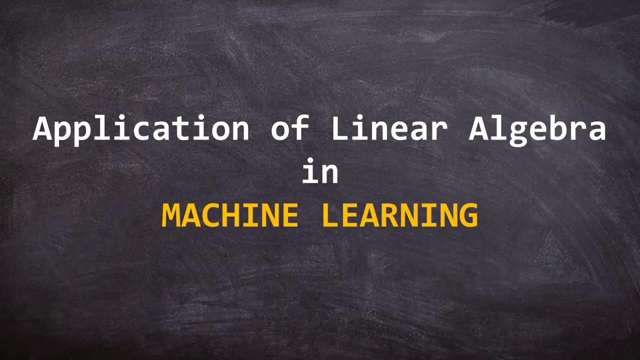 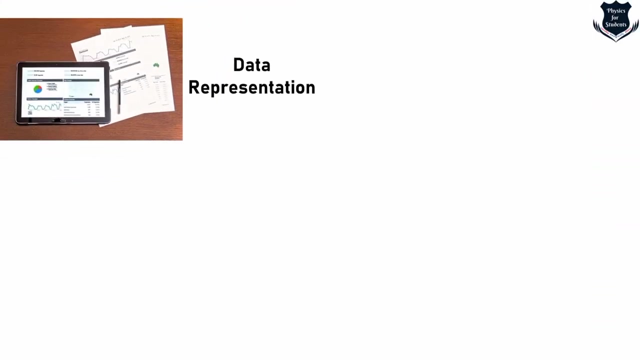 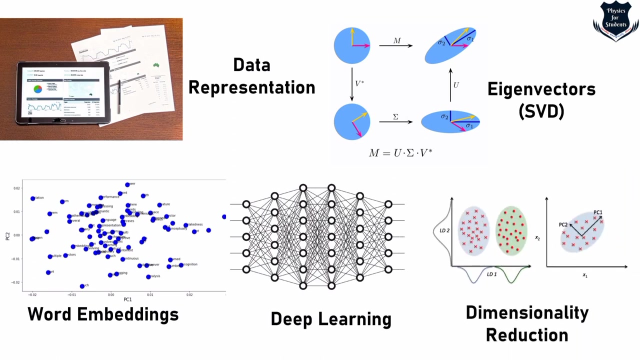 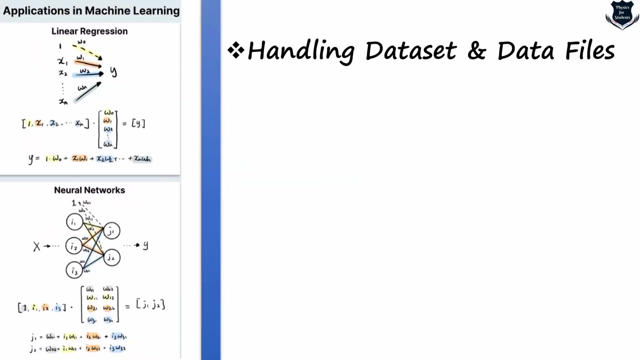 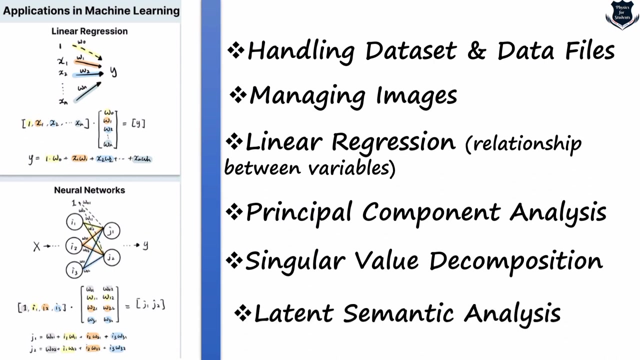 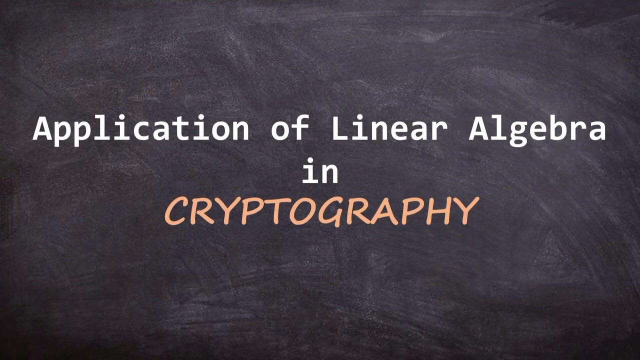 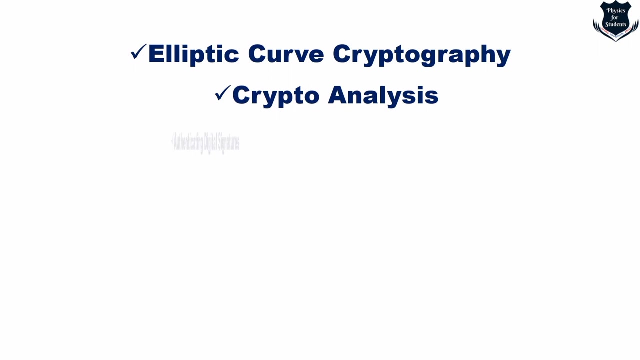 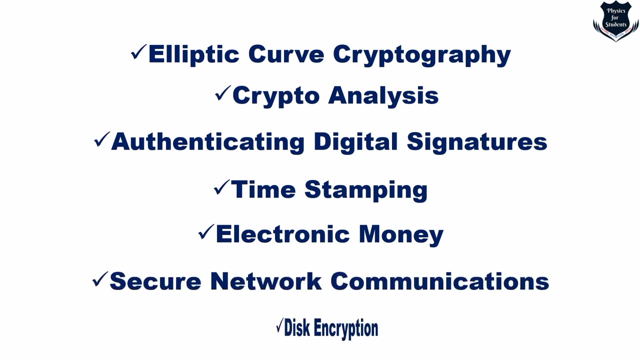 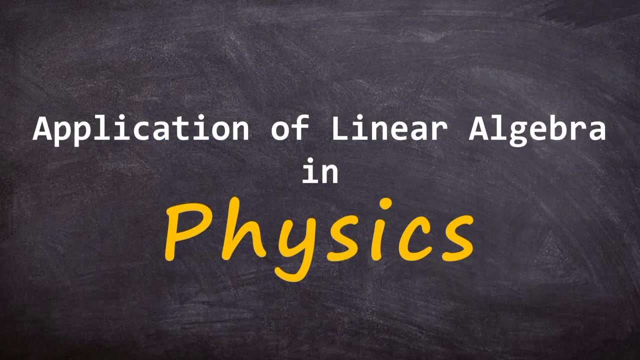 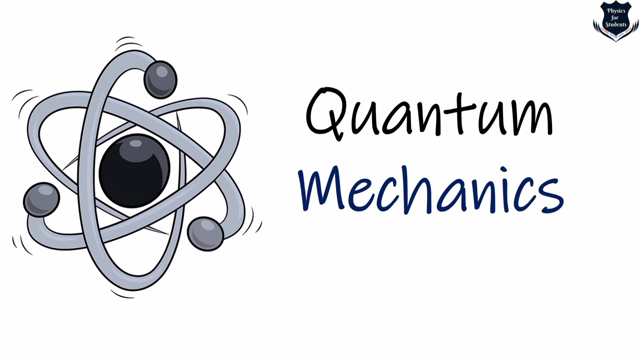 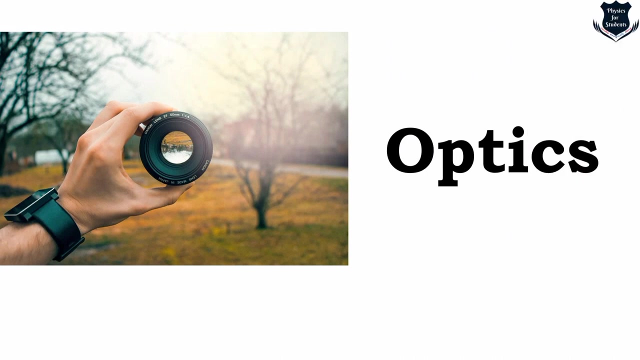 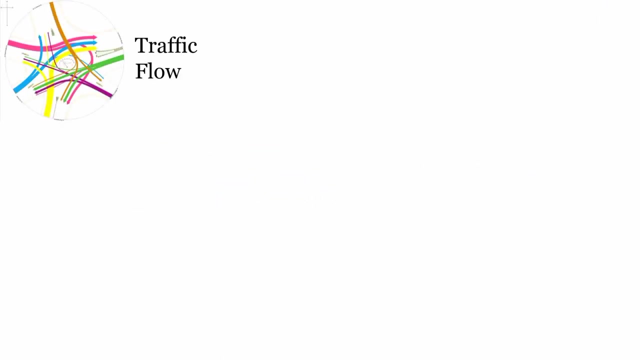 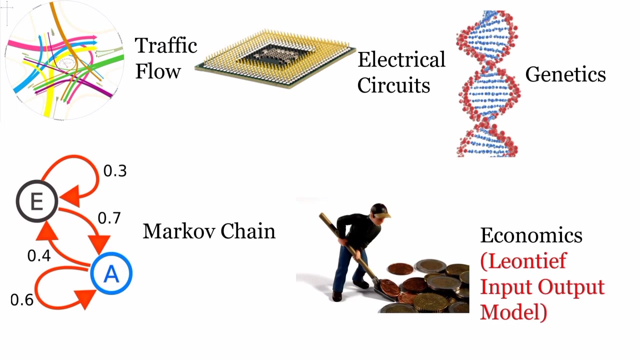 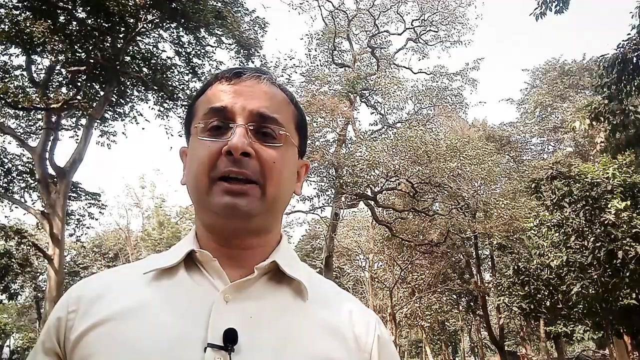 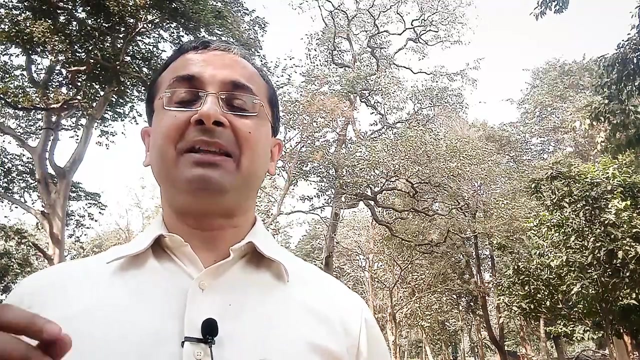 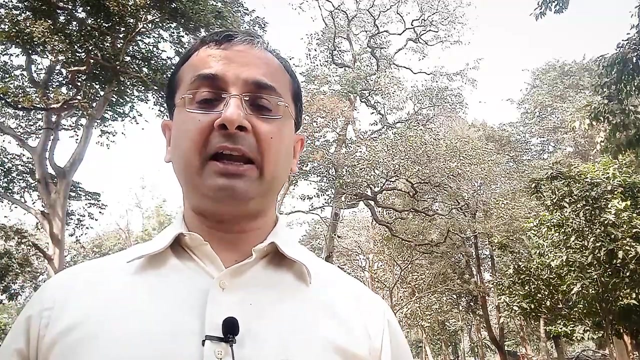 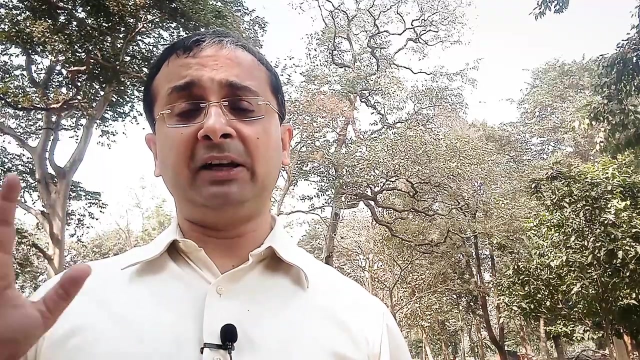 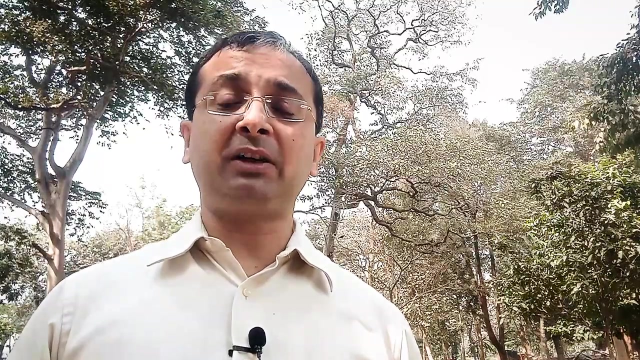 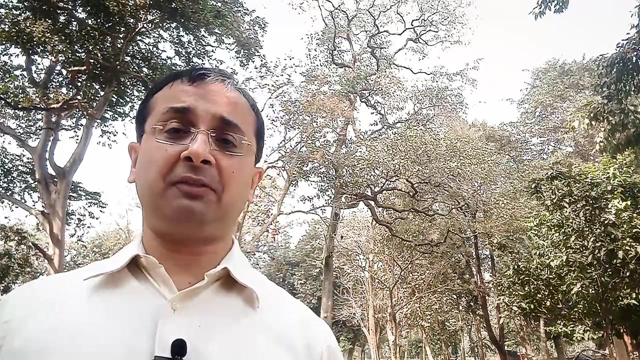 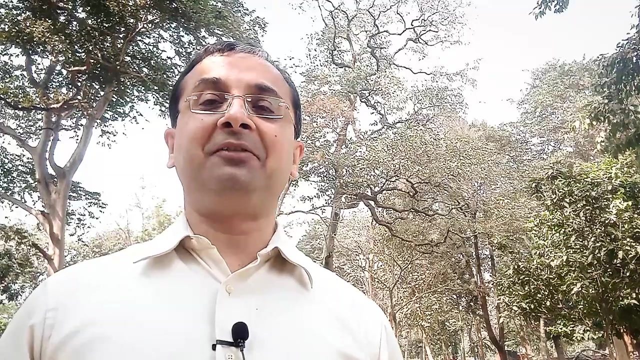 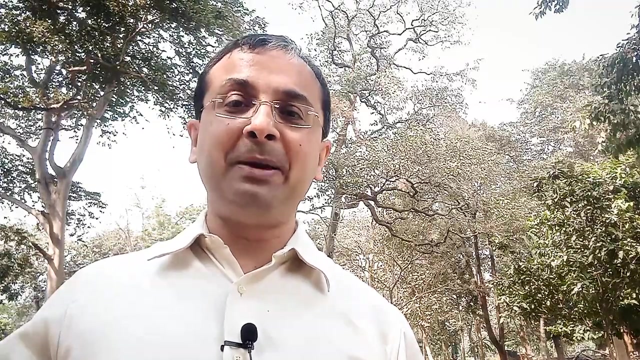 difficult to decrypt. so the encryption, as well as the other way of decryption of the data, is being done through linear algebra. so so, so, so. so I hope this video has given you a motivation and inspiration that when you are seeing those matrices and vectors and decomposition and hermitian matrix, don't worry. there's a big, big science.